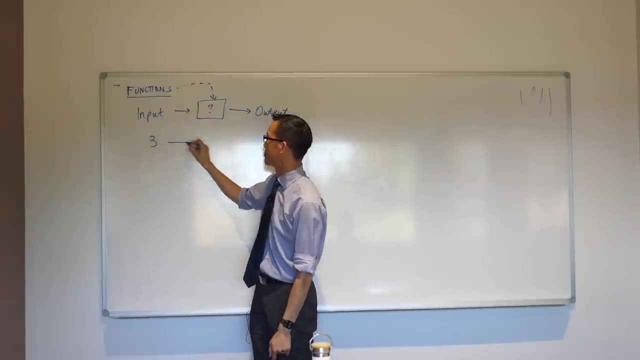 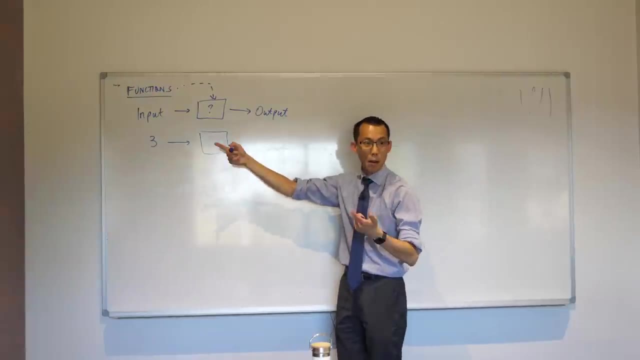 If I took a number like say three, and then I said, hey, the thing I want you to do, this, this process I'm gonna ask you to do, is to multiply that number by itself. right, We have a name for that process, right? What would you call that? 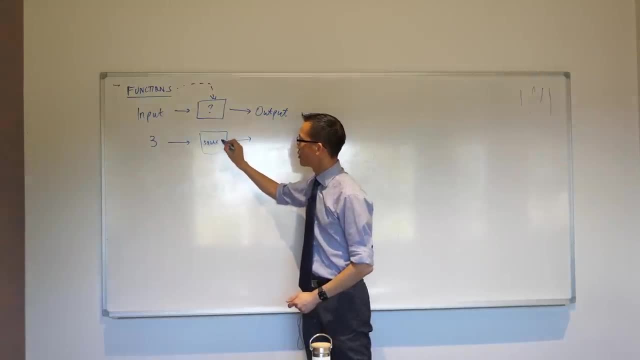 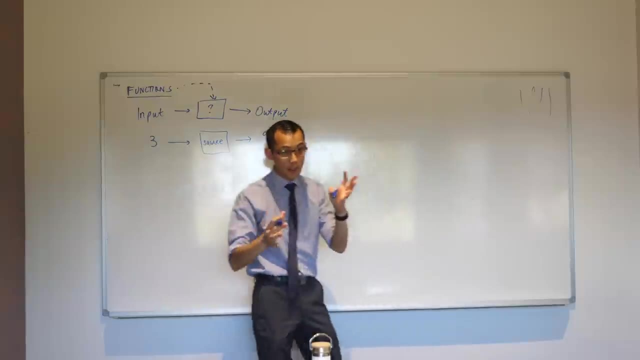 Squaring right. So we might say: this is a function that squares things and you get an input. you get an output which is, of course, Nine. Okay, happy times. This is a very simple function. Let me give you a slightly more complicated one. I might. 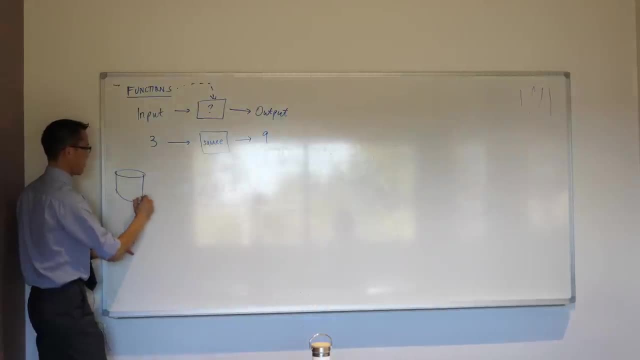 say: hey, we've got a shape here. right, Here's a cylinder. okay, Now if I wanted to work out the volume of this cylinder, there's two measurements that you need to know right. Firstly, you need to know how tall it is. What's the other? 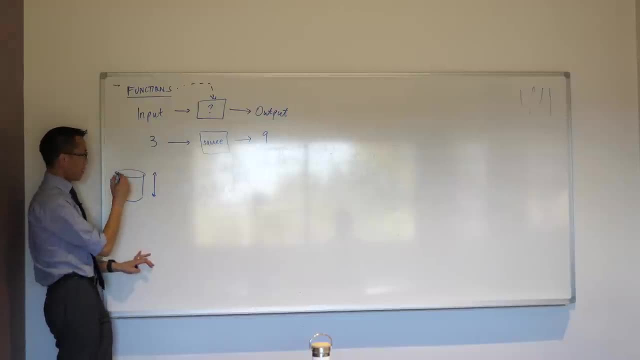 measurement. you need to know, Okay, so it's gonna have to do with like: this is just sort of like a flat measurement, but you need to know something about this right Now. if you had that area there, what you could work out, what you could. 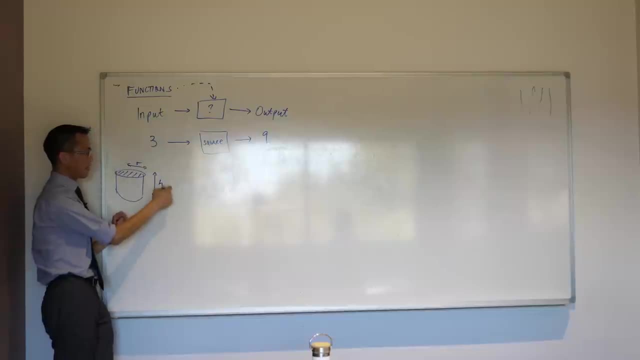 use that to work out is the radius. and then with these two things- see, these are inputs. so I'm going to say r and h, the radius and the height- you would put that into a particular kind of function for the cylinder. it'd be the volume function and then you'd get a. 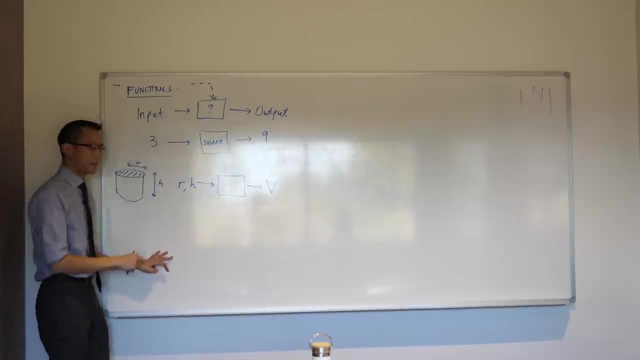 volume at the end. okay, Now, in this case, do you actually know what the volume of the cylinder is? I picked something out of random, that's okay. The volume of the cylinder, or maybe, yeah, The formula. Yeah, just the formula, I'm pretty sure I'll give you, I'll give you a clue. Starts with a pi, because it's a circular thing. 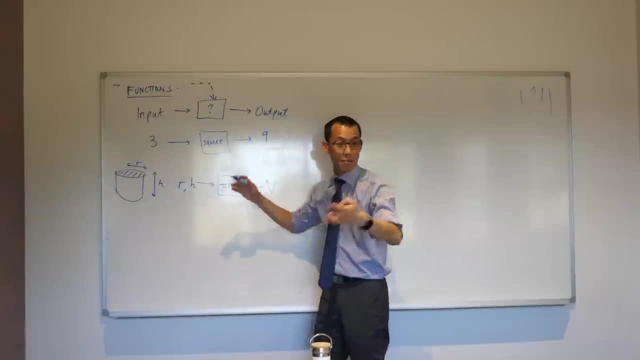 Pi r squared h: Yeah, yeah, yeah, Perfect, bam, okay. So what you've got here, right, What you've correctly identified, is here's a formula. all you need to do is take whatever those values are, substitute them. 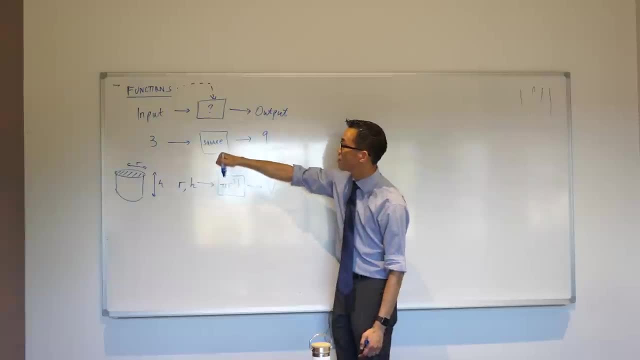 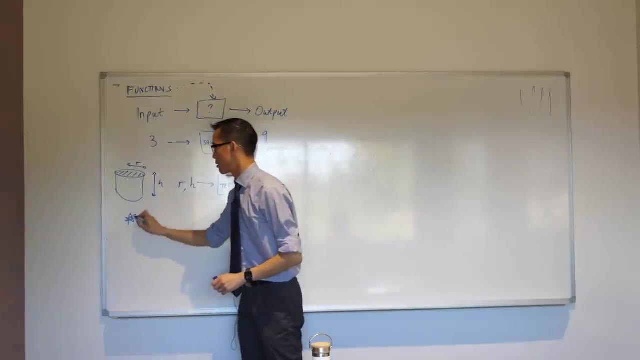 in and then you get some answer at the end. So these things here in the middle, these are the functions. okay, So let me introduce- and this is worth writing down right, Let's introduce- a bit of notation, So, because these are all called functions. 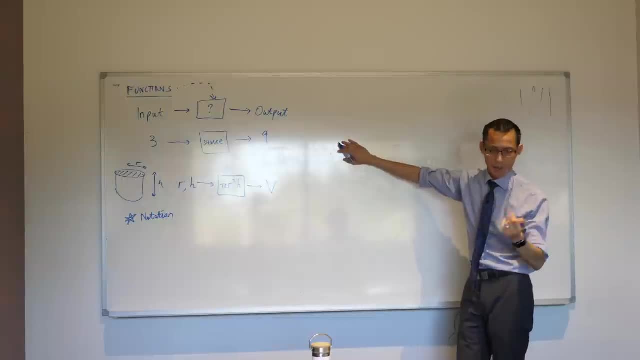 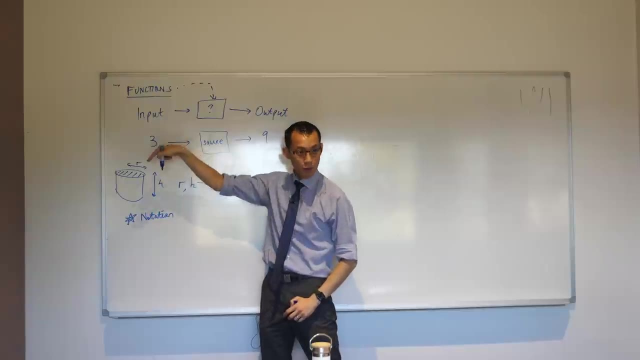 we use the letter f a lot and it just abbreviates function, right. So this one here, right, This thing, that's squared things. I might say, okay, this is the input and this is like your, your x value, okay, This is what you're going to put in. and then this thing: 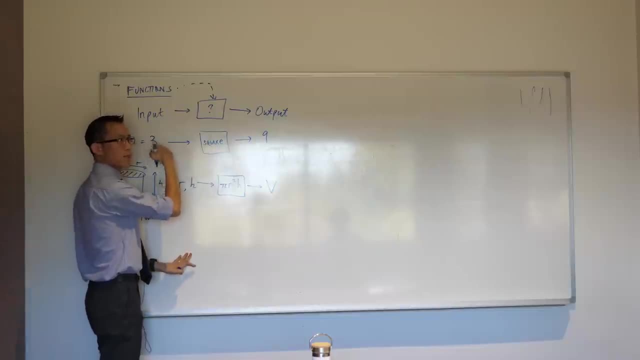 here it's like: oh, it's just you take that number and you multiply by itself, So you would write that as x squared. okay, So the name of this or the way that we would denote this. 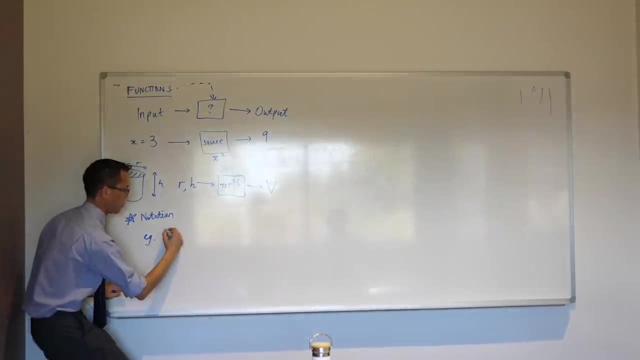 and you might have seen some of this in the textbook is, I would say, for example, f with a bracket: x right equals x squared. Now, super important to just pause on this for a minute. Have you seen this before? 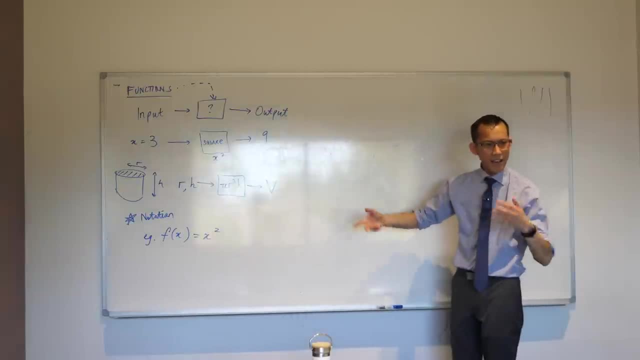 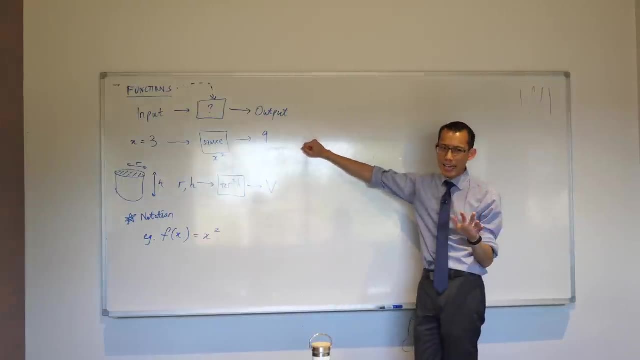 Yeah, Yeah, Okay, I caught a glimpse of it. Yeah, yeah, Yeah, sure, Now I. I just want to hover on this for a minute because mathematicians really lazy. they want to write things very succinctly and efficiently. 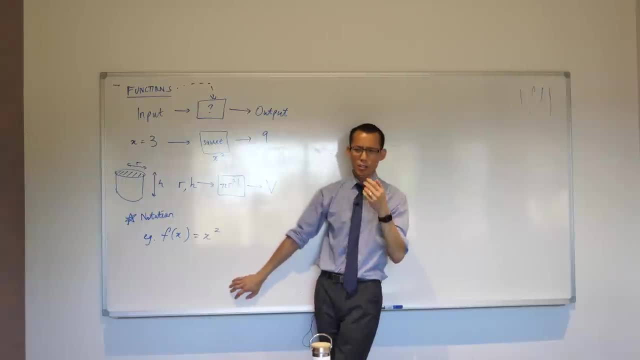 but for that reason, sometimes they will. you know how in English? I'm trying to think of a good example for you, right? In English, sometimes a single word means two things at the same time, and you have to work out, based on context, which one it means, right? So 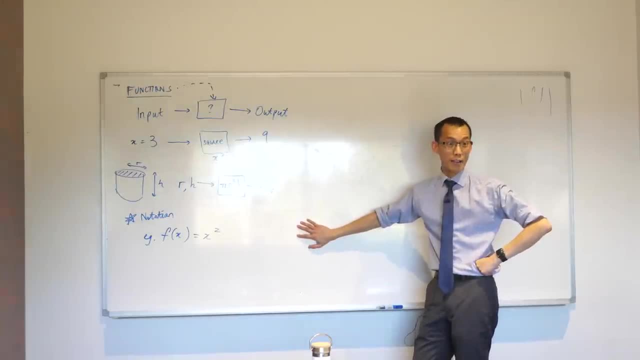 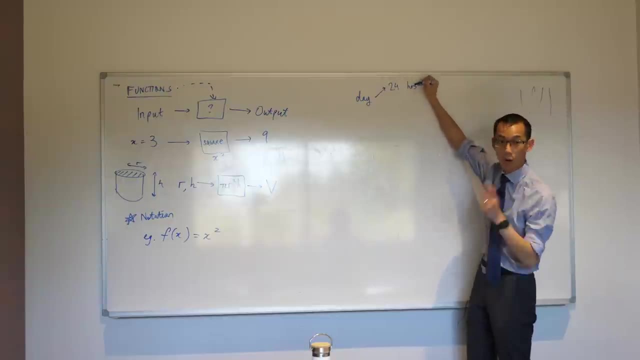 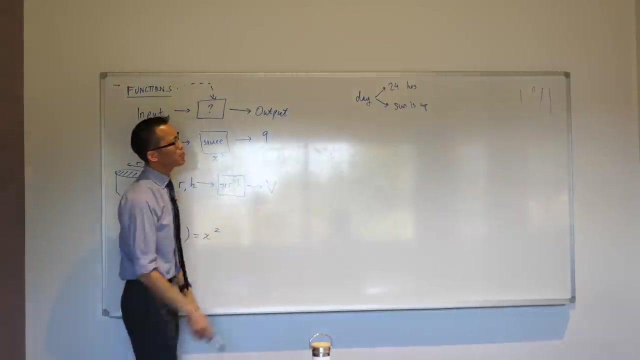 if I said the word day d-a-y, right, You're like: oh, do you mean that's 24 hours, Or do you mean just the time when the sun is up? Now, those are related but actually quite different, aren't they right? Night and day versus days, months, weeks, etc. How would 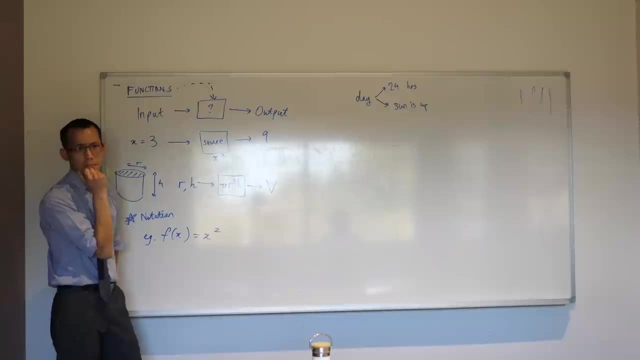 you be able to tell: Um, it would depend what was in front of it. Very good, Yeah, it just depends on, like this context around this that indicates to you. okay, Now the exact same thing is happening here, If I didn't give you any context. 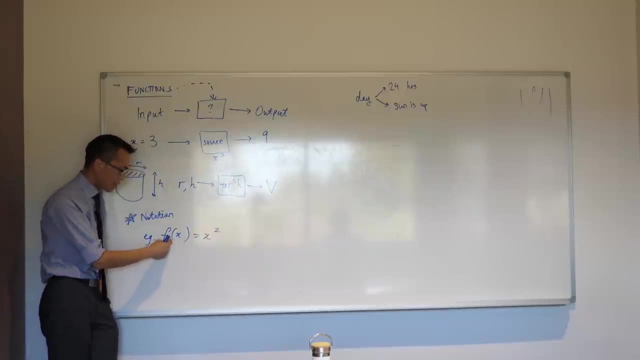 whatsoever. and if I said there's a letter and then brackets and something inside, if, for instance, I gave you something like this, This probably suggests to you like that there's an operation that you would do between these. What would you guess the operation? 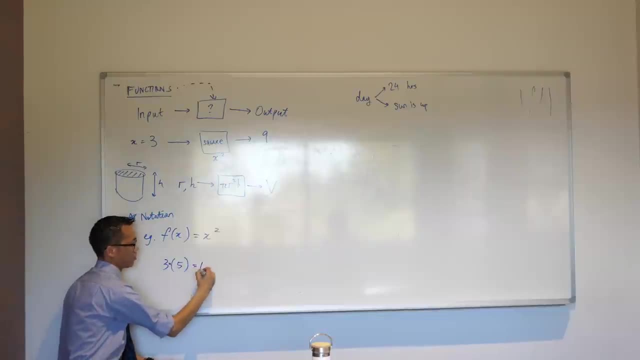 is: Yeah, multiplication is kind of implied there, right? So in this case you just say: oh, 15,, right? So the context here of numbers tells you it's multiplication. But here, and particularly the fact that they use this letter f, they'll use other ones as well. G is the. 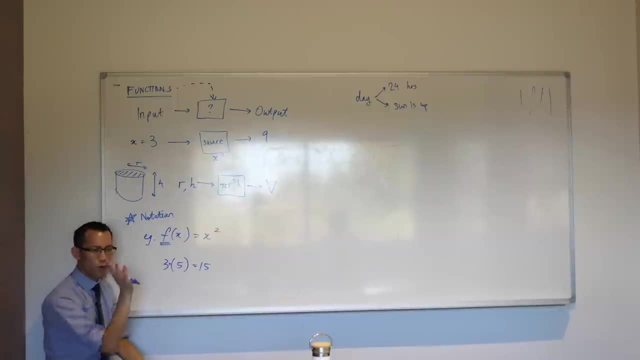 letter after f comes up a whole lot. Sometimes they'll use u or v, But this context tells you there's not multiplication actually happening. This is a name of a function. I'm just going to call it f, And the thing it tells you to do is square things. okay, So that's one. 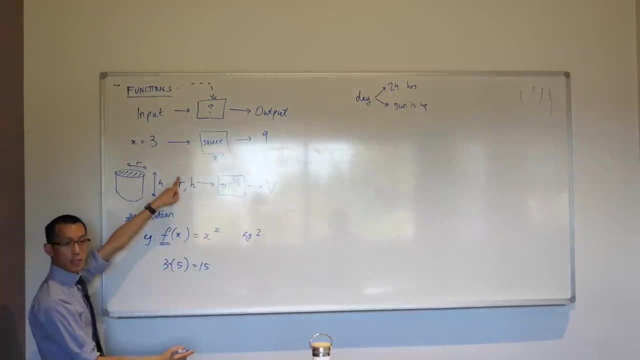 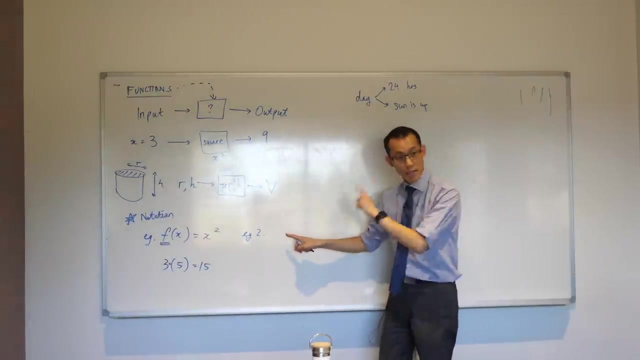 example. Let's give you another one. It's this one that you just did here, right? So this here is a function that does what. What did it? Do you ever see it? Very good. So in this case, you would say, well, why don't we just call the function like a name that? 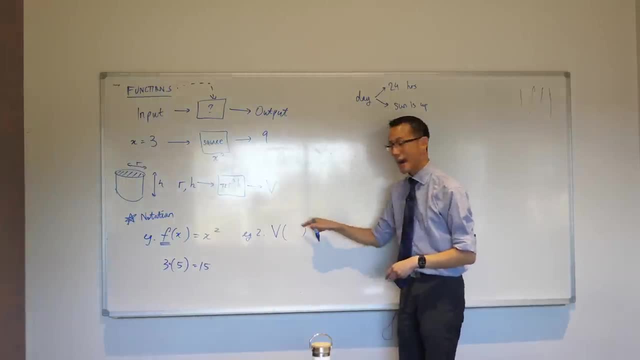 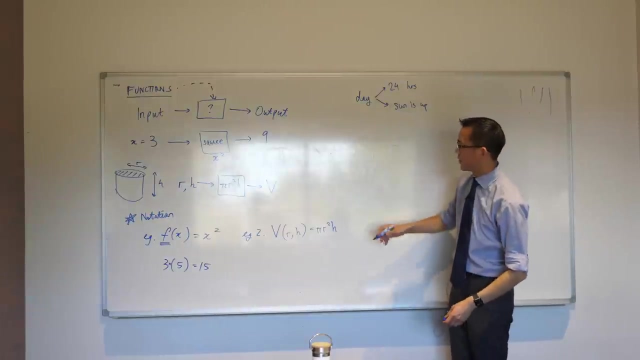 is a bit more descriptive, right? And then what you put in these brackets are the thing that goes in. It's the input, right? Very good, So it's r and h, And in this case it would be pi r squared h. okay, Now I've given you. 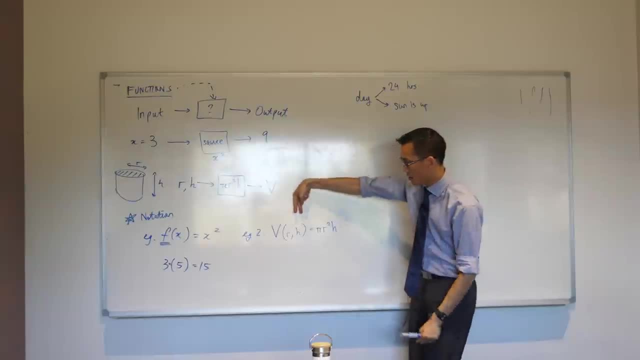 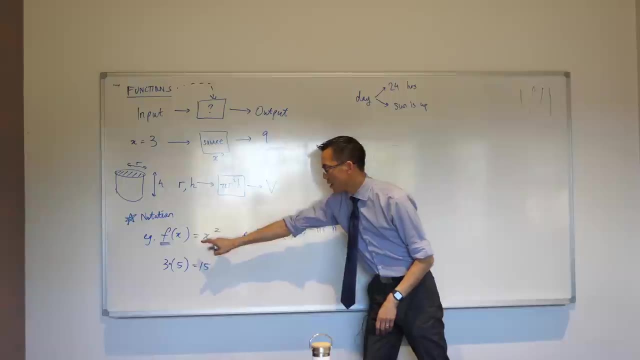 these kinds of examples here, because the basic idea is just there are inputs, Inputs. You do something to those inputs and you'll get some answer at the end, Like, say, 9 or I don't know if this was a radius of 10.. I'll write this down: Radius of 10, a height of 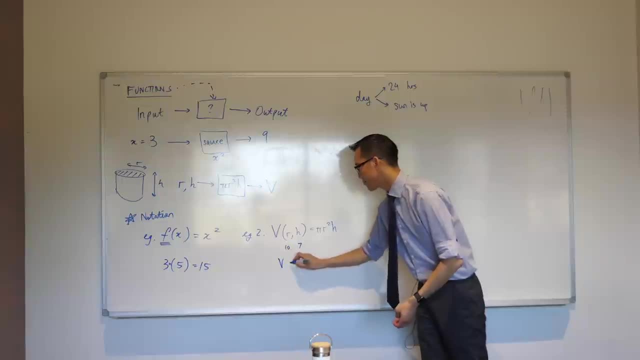 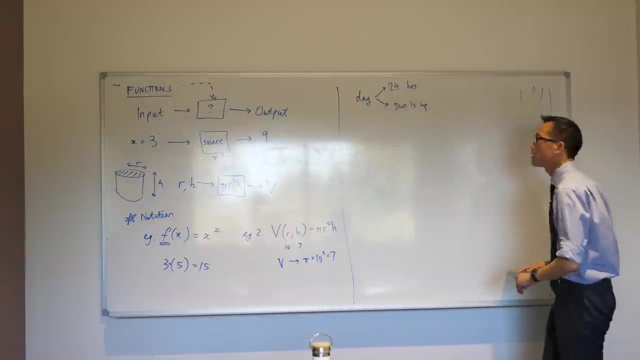 7. Then my volume would be equal to pi times 10 squared times 7. 700 pi. Does that make sense? So there's inputs, there's outputs. okay, Now, nicely for you. just realize I didn't bring in a whiteboard eraser. I'm going to get one in a second. Lucky for you see. 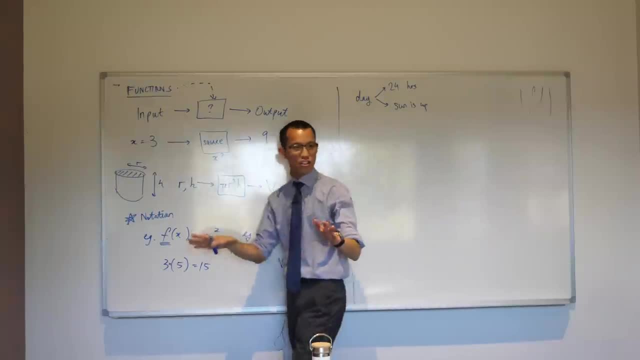 how this function has two inputs. We're pretty much exclusively going to stay in the realm of functions which have one input And actually, if you just have a look, you've got the textbook open. yeah, You're going to see, and I want you to give me an example, actually Give me an example of a function. 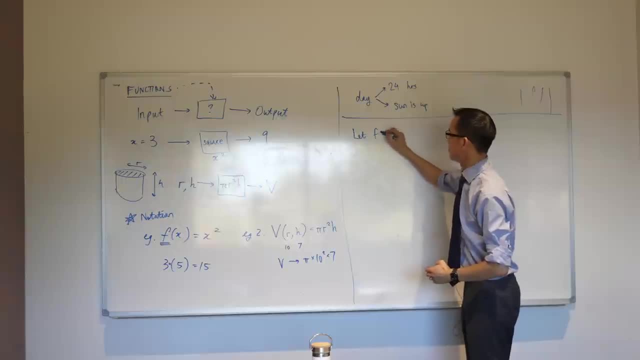 they're giving you. Let f bracket open. bracket x equals bracket equal 2x plus 3.. Great, Okay, So you can see all of the pieces of the puzzle we mentioned before. right Are in here. There's a function. It's just called f, Not very original The input number. 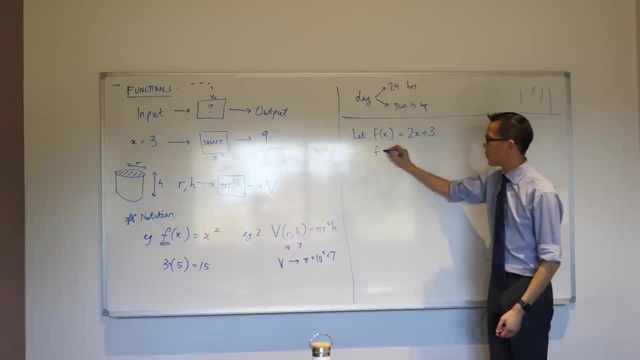 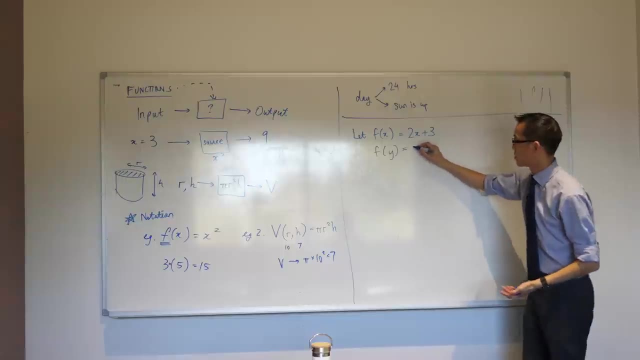 is here And, by the way, we don't have to call it that. We could have had f of see how I had radius and height. I could have. I might have an input that's like y instead of x and it would be you put. 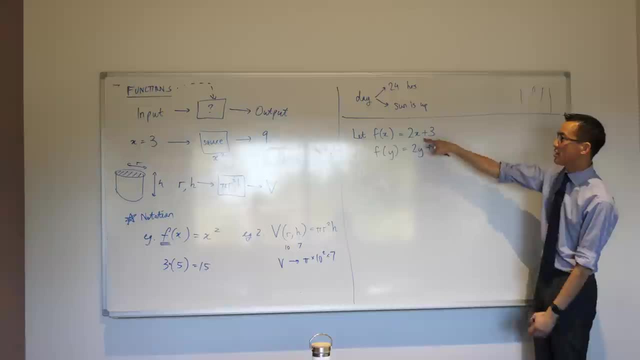 in y's instead of x's. okay, And then this is the. this is the box. This is the function that does things to the number. okay, Now what's it asking for? Like they said, this is the function. What have they then asked you to do with that? 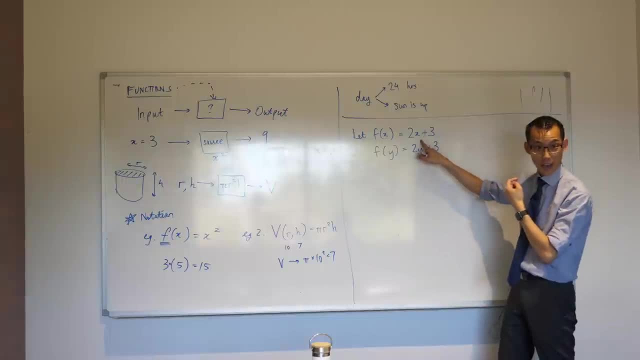 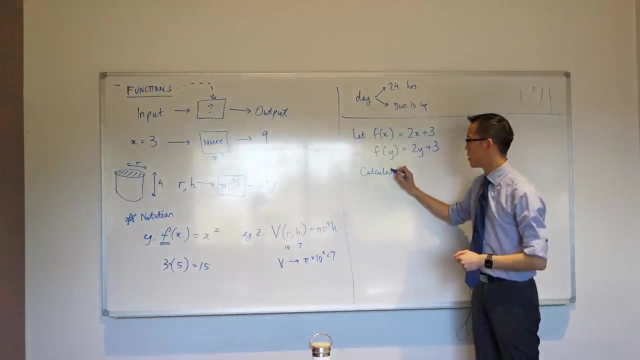 Value of x. Say that again. Value of x. They want a value of x. Read See, does it? oh, yeah, Calculate, Yep, So you have to find x and then put in the equation. Yeah, So you have to find x and then put in the equation. 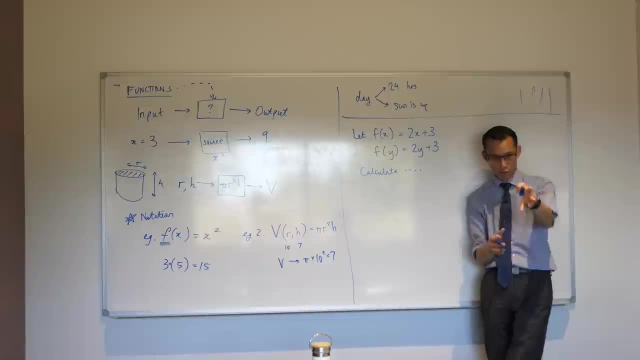 Yeah, Okay, very good. So they would say: calculate. and then I presume, I'm guessing- they're going to give you different values of x, and then they want to know what is the? what's the output? Yeah Right, Can you give me an example? What's, what's one of the values of x they want you? 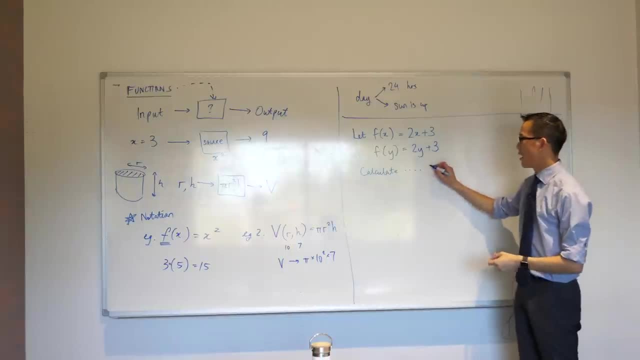 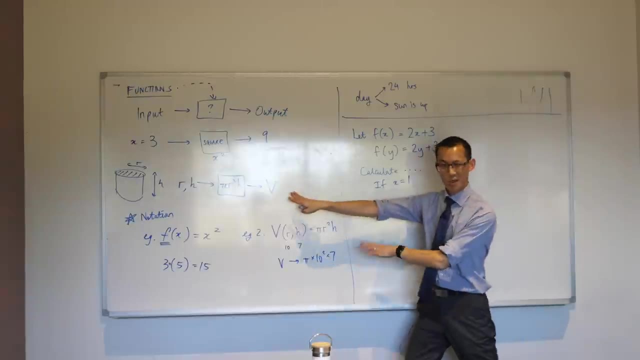 to do. The first one is one. Okay, So if they said, if x equals one, right. So the way we would write this again- I'm trying to introduce the notation to you- is we would just put that one wherever we. 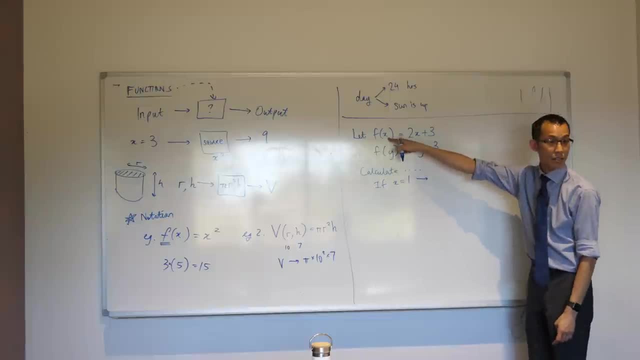 see x right. So that would literally lead to: well, the first x is right. So I'm going to say, and I read this as f of one, In fact, you know what this reminds me of, and I wonder if you recall this from years ago, maybe three years back, Do you? 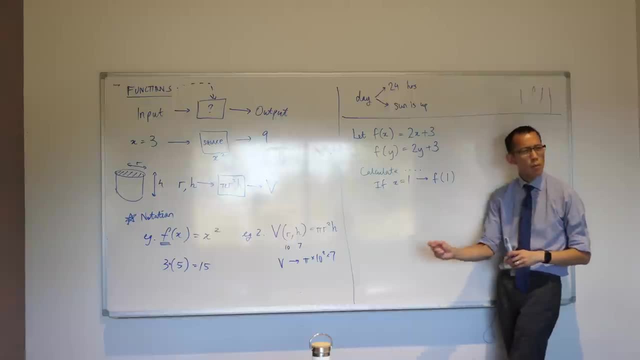 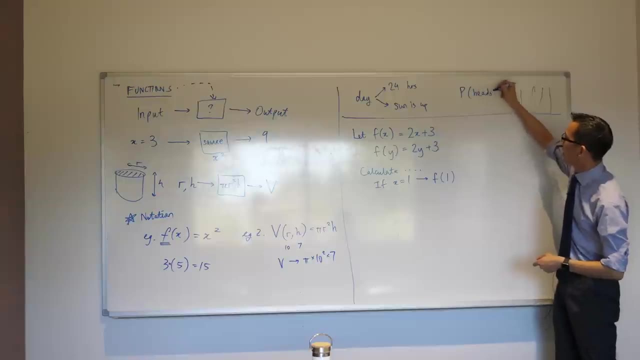 remember we used to do. well, you'll later on you'll do some more probability, like rolling dice, stuff like that. Did you ever encounter this? Yeah, Like like heads or tails or something like that. right, That's when you're writing the probability. 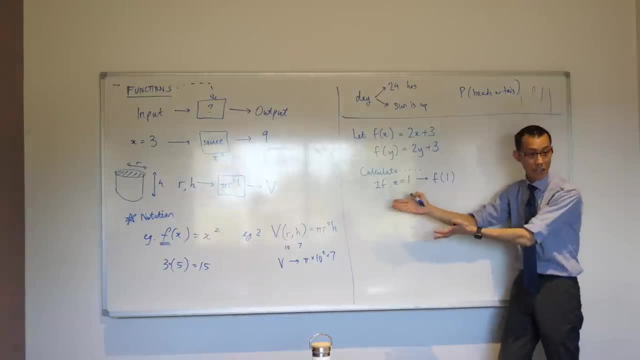 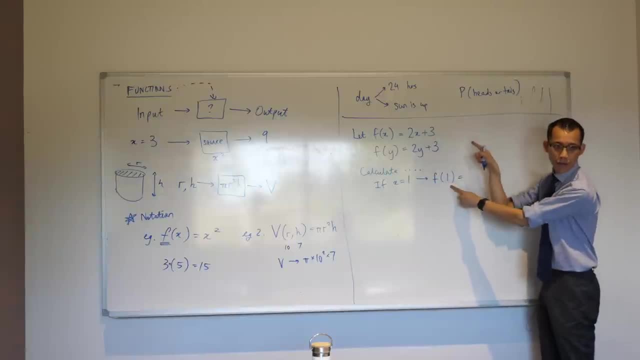 I'm actually just going to put in one wherever I saw x. okay, So I'm going to go two- there's x right there- plus three. Can you evaluate? for me, It would be: f of one equals two plus three, which is five. 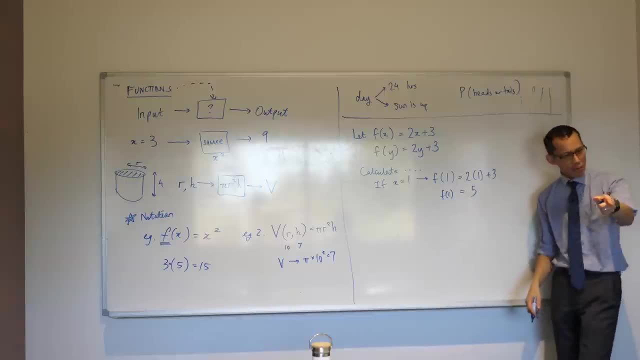 Fantastic. I'm just going to go straight to five. I think we can handle that right. So that's really good, Well done. Now it's really sneaky, right. Even just in one line we're using this notation kind of differently, right, Because you knew correctly that that 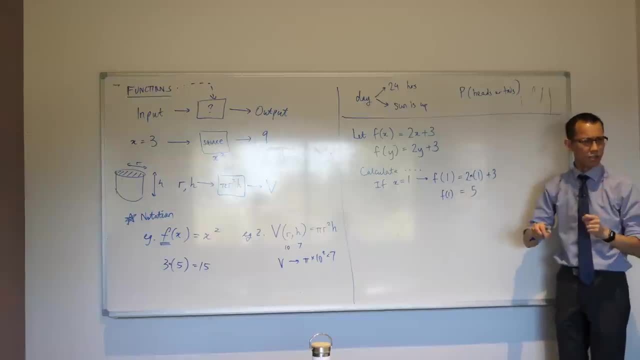 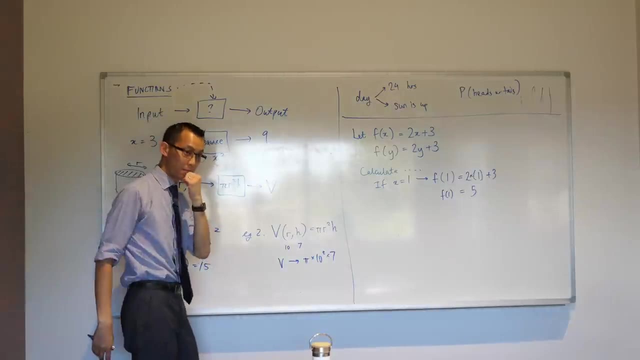 was multiplication, but here it's function notation. okay, Did you have a question just there? Oh no, I was just quizzically looking at it. Yeah, It's a bit funny. okay, Did they give you another number? Like we've got x equals. 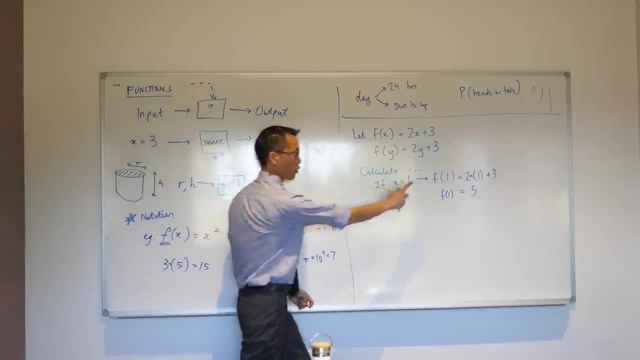 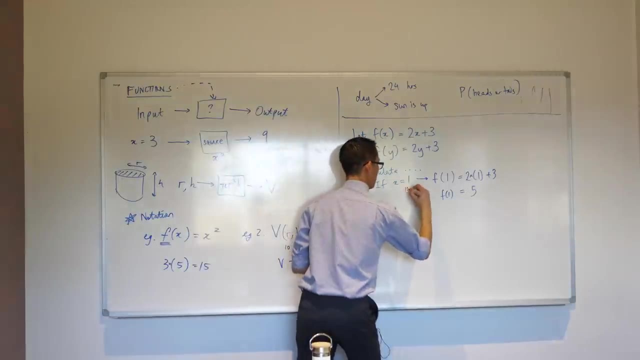 one. So that's the answer, That's it. Oh, okay, That's it. That's all there is to it, right? So the input's here. In fact, I might just highlight that. Okay, Okay. 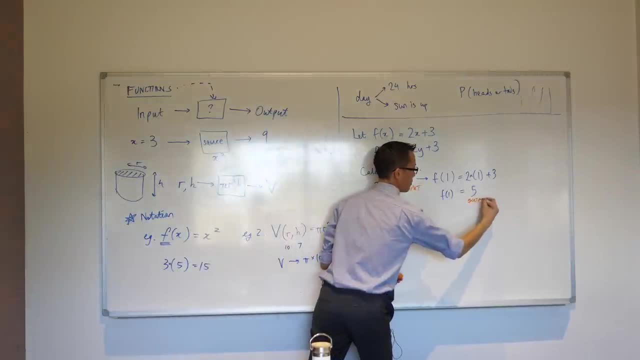 Okay, Okay. And here's the output: Yep, And in the middle is the function slash process. Yeah, That's right. This here really is that function Or, like you said, it's just a process with some algebra. 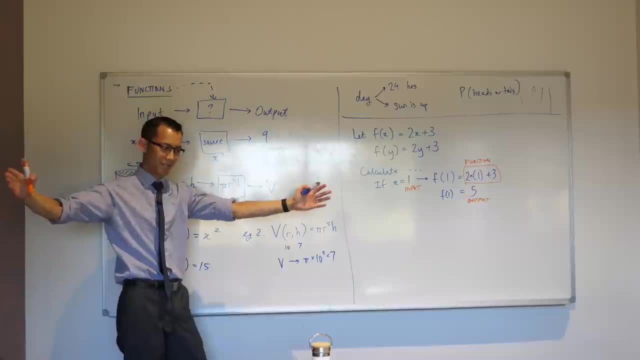 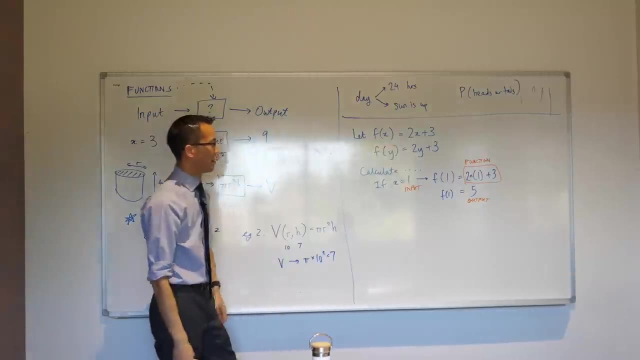 Right, And you can put anything you know in there. So over the last 11 years you've learnt you could put in square roots, You could put trigonometry, You could put logarithms- Any of that stuff can fit in here. 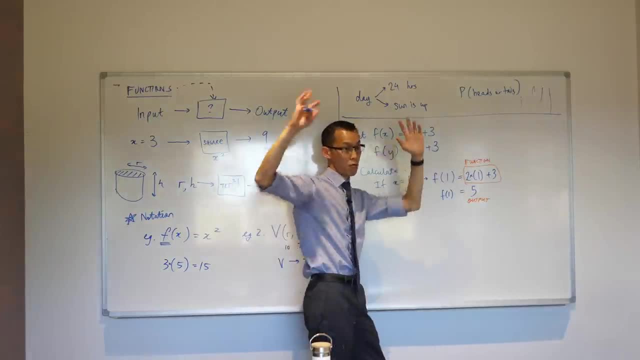 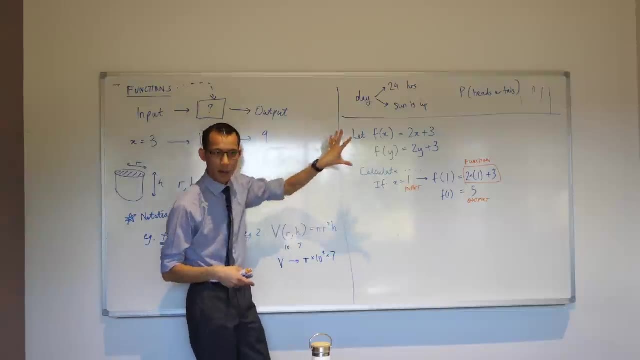 Yeah, So that's the function. That process is very, very broad. It can include anything. Okay Now, just before I ask you to give me another example in a minute, I actually just want to press on this example for a minute. So you see how we said: if x equals one go. 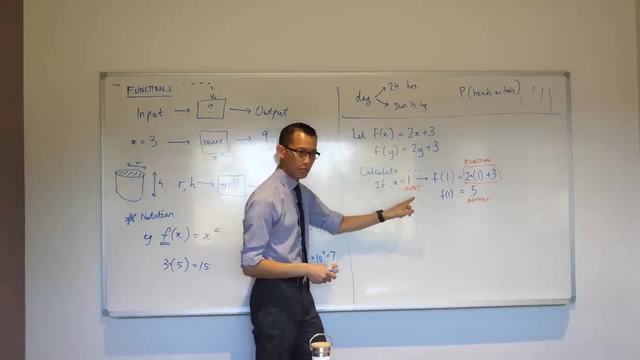 ahead and work out the output. Right, You can make x equal to anything. So, for example, I want you to see if you can help me work out here. Right, If I said to you what if we made x equal to not a number but a number. 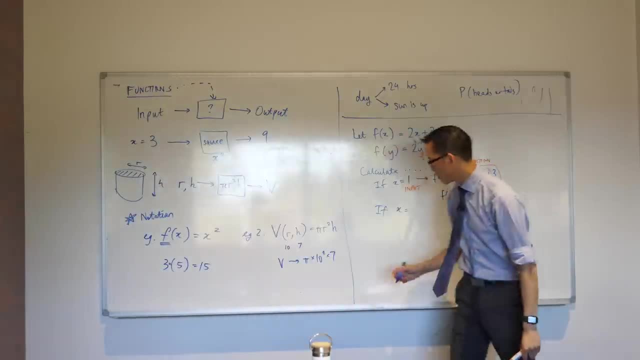 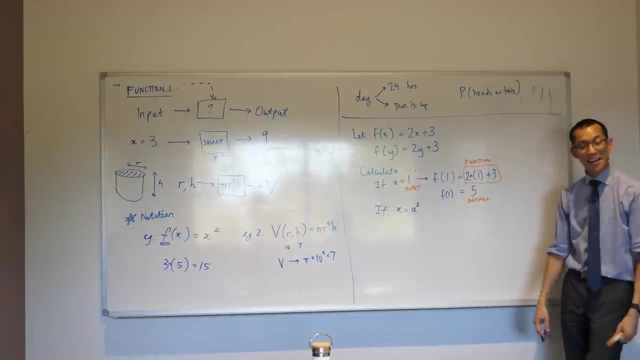 Another pronumeral, Another pronumeral, Right, Yeah. So for instance, I could put in, say: for instance: let's be, let's be a bit weird here, Let's put in a squared there, Oh God. 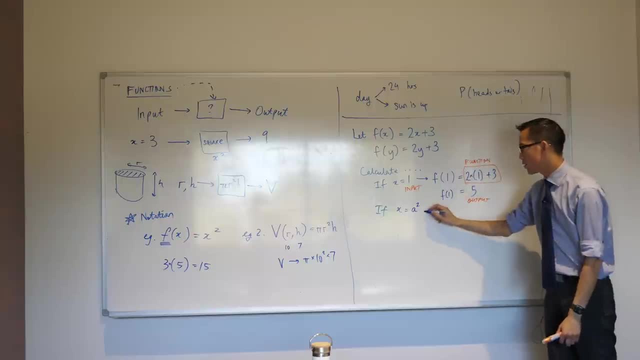 Now you don't need to fret, because they've given you a pretty easy example here, But I'm going to do- and I wonder if you can help me here- right, I'm going to do exactly the same thing I did with one. I'm just going to do it with a squared. 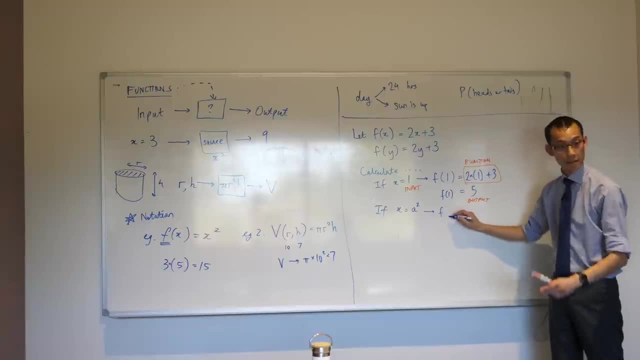 Okay, So it's still going to be two of something plus a. Yeah, that's right. So just before we get there, right, I'm going to write it from the beginning. So I'm going to write f of what. 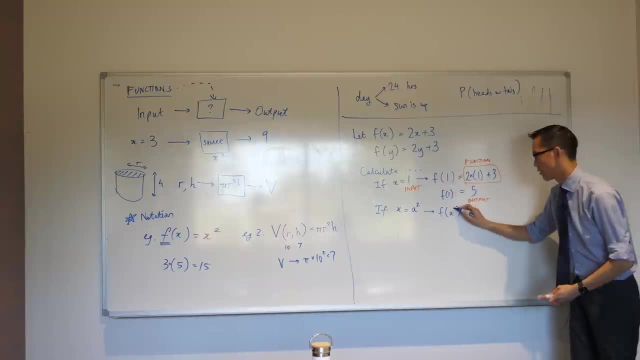 A. A squared Right Exactly Equals Two, Two Of a squared, So two a squared, It's just two a squared, yeah, Two a squared, plus three a squared, Ah, Three, No, no, Because there's no bracket. 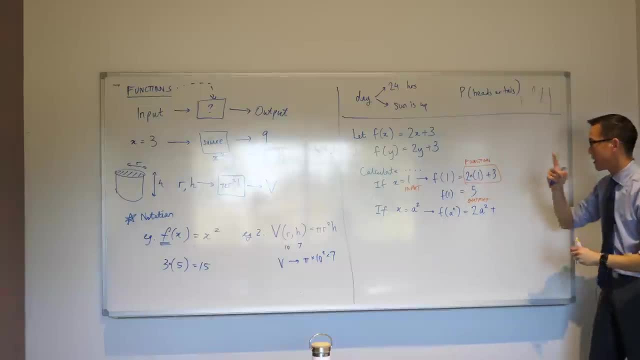 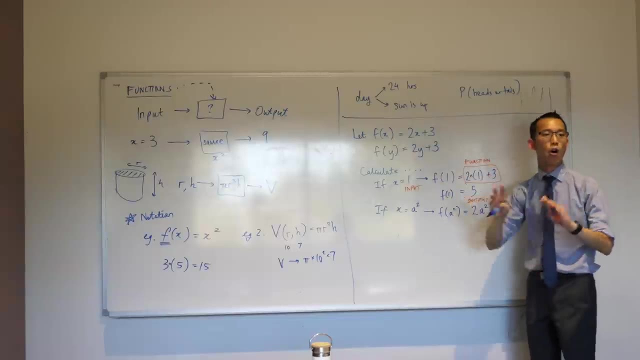 Yeah, I'm so glad you actually said that, because this is the pit where it's like: oh yes, where do I put this a squared? And the answer is: anywhere you see x, and only where you see x. So it actually is a very common thing to say like: oh, do I put another thing here? 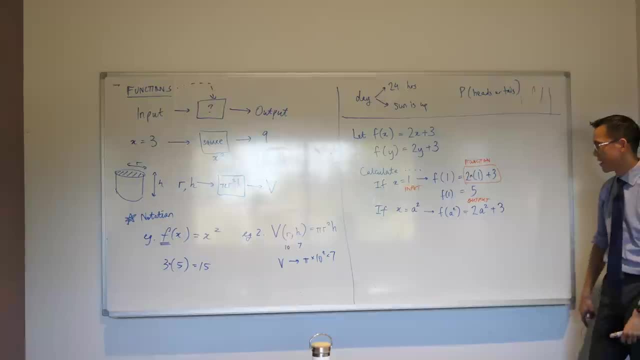 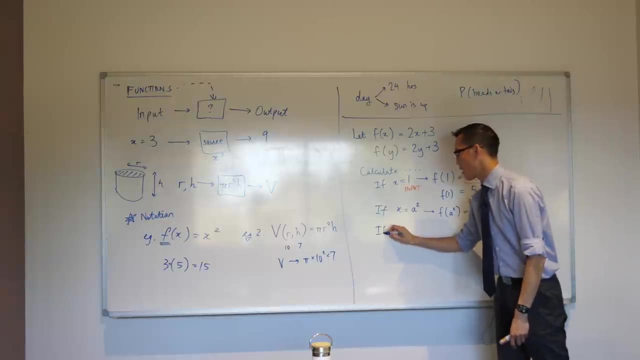 And the answer is no. that three just sits by itself. Yeah, Okay, Let me give you. that's right. It's like, oh, I instinctively put stuff there. Let me give you one more example. Okay, Let's see how you go. What if x were equal to? let's. 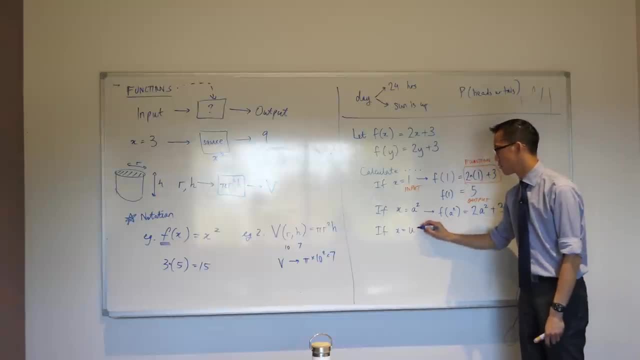 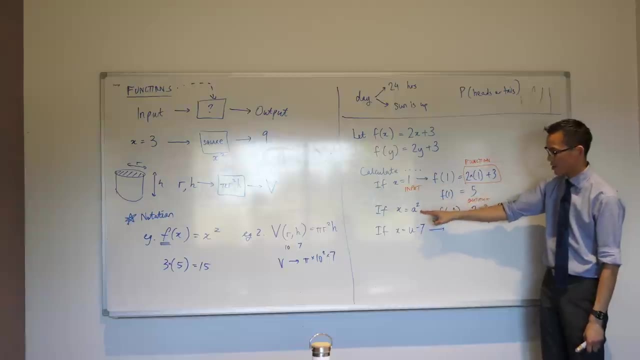 do this. Let's go, u take away seven. Okay, Now here it's not just a number, It's not just a single algebraic term. I've given you like a few things, right, So it's going to. 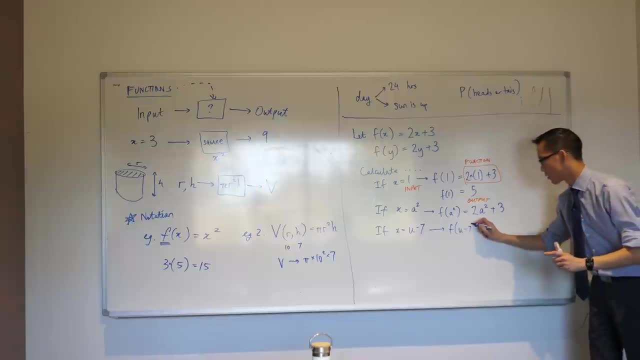 be f of U minus seven, U minus seven, Great. And then what It's going to be two? u minus two, u minus fourteen, Oh, very good. So you've- actually you've- expanded all in one hit. That's great because 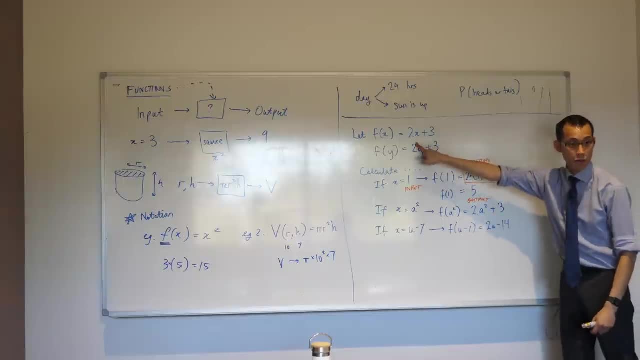 what you did was the whole thing was multiplied by two, which is perfect, right. And then what? And then mark plus three, Very good, So that plus three just kind of hangs out on the end. In fact, what you'll. 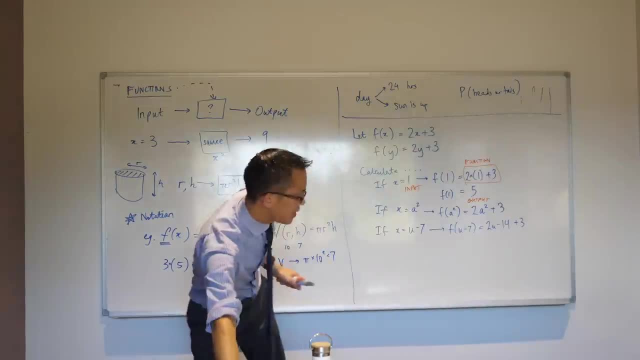 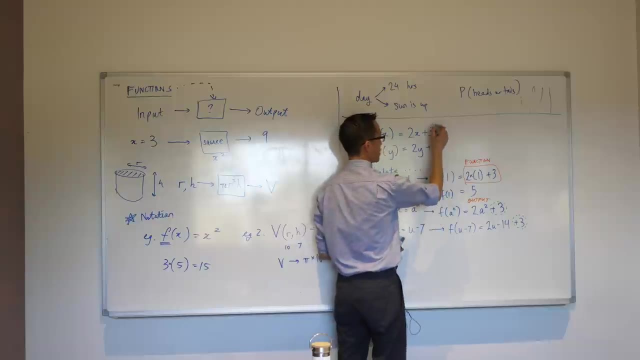 notice- by the way, let me get a new color- is that plus three is kind of it's. it never changes, right It's. it's sort of like, no matter what you put into x it never, it never.